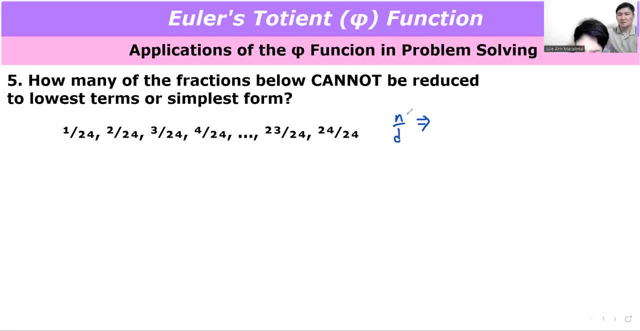 So for any fraction N over D, where of course N and D are integers, are already in simplest form, It means that the gcd of n and d is equal to 1. It means they share no common factors. Yes, Which is the very definition of the simplest term to be in simplest terms. 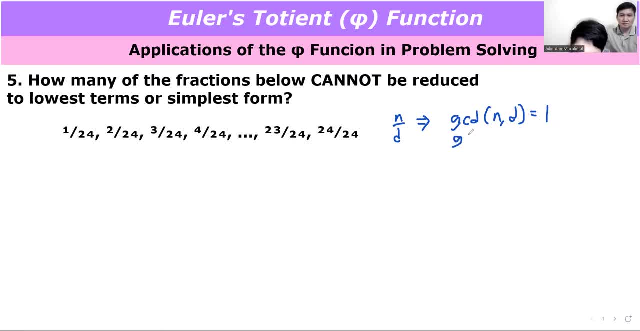 So in this case the denominator is 24, so we can already point out that the gcd of any numerator of these fractions, in already simplest form, is of course 1.. Okay, So now to solve almost any gcd problem we have to write out first the prime factorization of 24.. 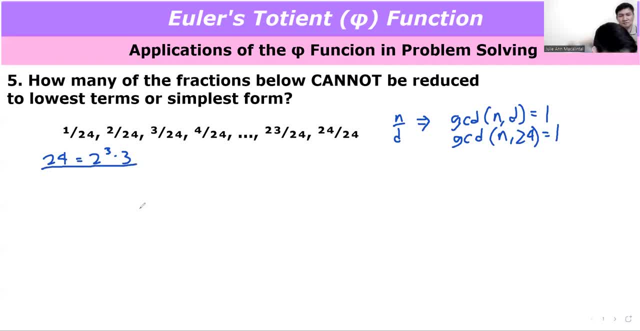 So I'll just put it here: Yes, yes, Okay, So phi of 24, the quotient function of 24.. Put it a little below. it looks like a fraction. Remove the remove the remove the underline The underline. 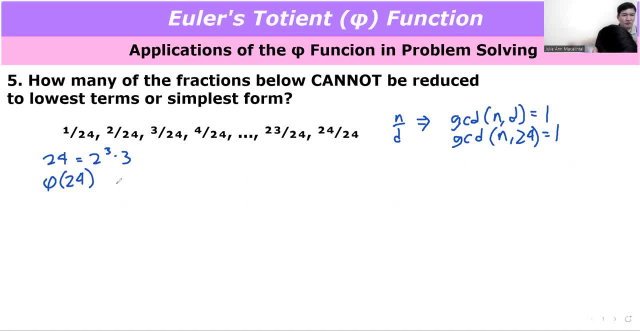 The gcd of 24.. Or the quotient of 24., Using one of the one of the one of the formulas that we have discussed in our video on the lecture about the Euler's quotient function. And then, of course, 1 minus 1 over E, n, which is the final prime, of course. 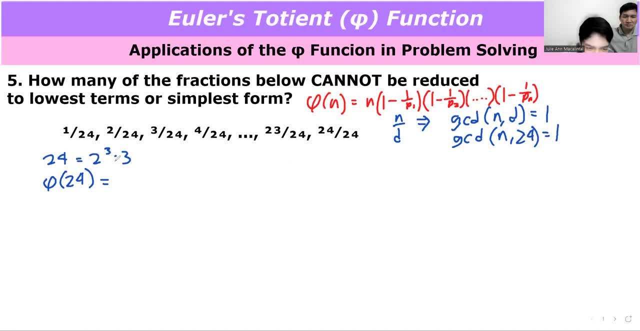 So here we will apply that We now already know. the prime factorization is just 2 and 3. So it's 24 times 1 over 1, minus the first prime, 2.. And then 1 minus 1 over 3, which is the second prime and also the last prime. 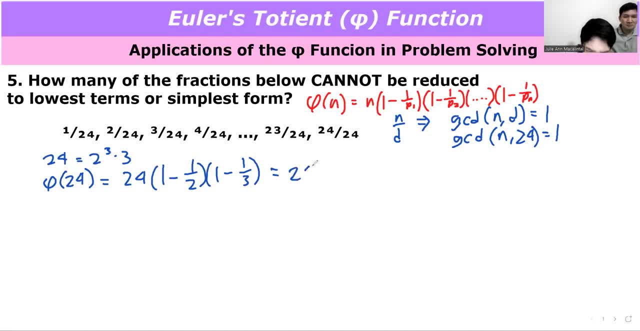 So then this is 24 and 1 half, And then of course 24 over 3 is 8.. So already we can point out there: 8.. And those 8.. What do you mean by the phi function of 24 is 8?? 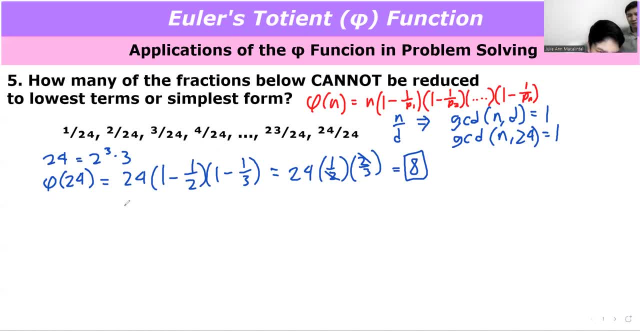 Yes, so those are the 8 totatives of 24, and I will write this down. Can you write the 8 totatives of 24 there? Those are 1,, 5,, 7, and 8.. 8 totatives of 24,, but those are 1,, then you do. 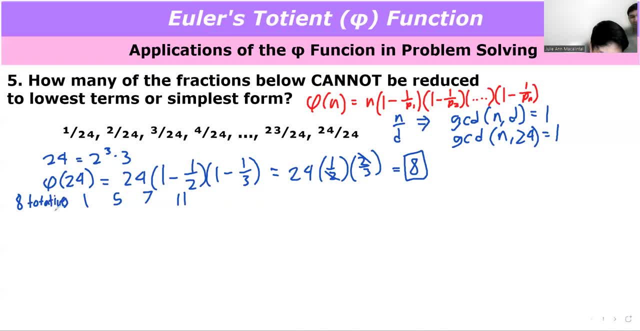 Don't assume 8 totatives of 24.. 1,, 5,, 7, 8.. Use a different color: 1,, 5,, 7,, 11,, 13,, 14,, 15,, 16,, 17,, 18,, 19,, 20.. 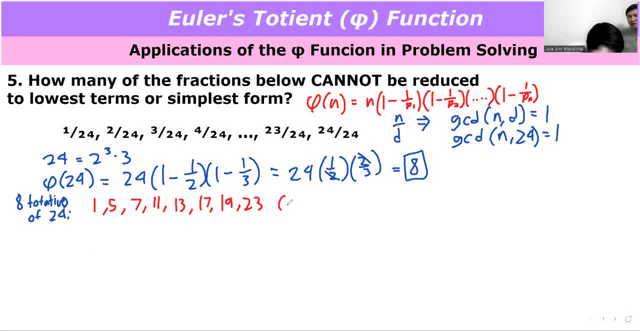 23. These numbers are relatively prime to 24. So of course they don't share. That means they don't share any common factor with 24.. And then 1 is a special piece, because 1 is counted as: 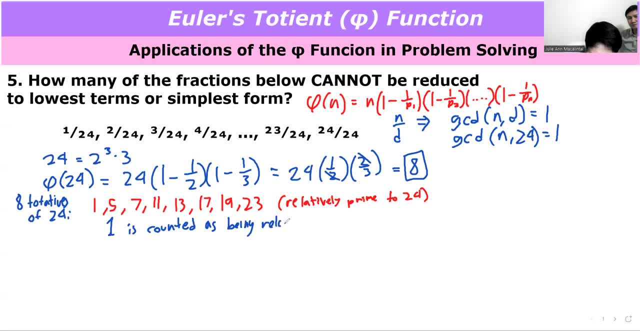 1. 2,, 3. 17. And 1 is a separate piece because 1 is a didn't have a positive term. 1, 5, 7, 8. 9,, 7,, 9,, 10.. 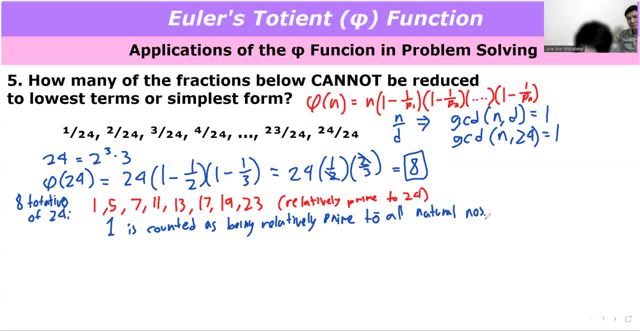 11. 11,, 12,, 13,, 14,, 15,, 16,, 20.. 21,, 15,, 21,, 22,, 23,, 24,, 25,, 26,, 27,, 28,, 29,, 30,, 32,, 33,, 32,, 33,, 34,, 35,, 36,, 38,, 40,. 31,, 31,, 32,, 34,, 45,, 45,, 40,, 41,, 42,, 44,, 45,, 45,, 42,, 45,, 45,, 42,, 47,, 41,, 42,, 45,, 42,, 44,, 42,, 45,. 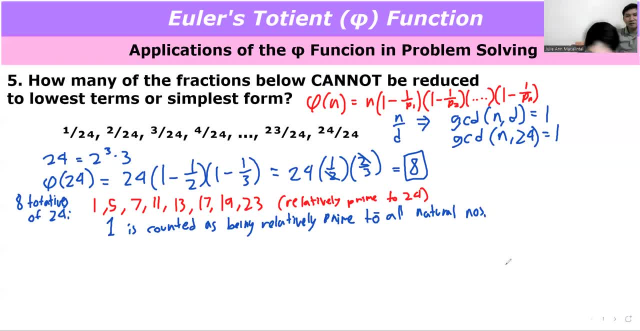 Yes, Yes, So that's it. So can it be reduced to simplest form or lowest terms, meaning you cannot reduce them further because they're already in their lowest terms and lowest terms, as Joshua pointed out, the gcd of the numerator and 24 is equal to one. these are the eight uh numbers, eight numerators, which. 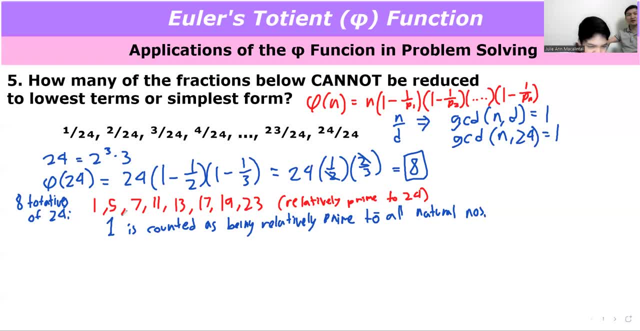 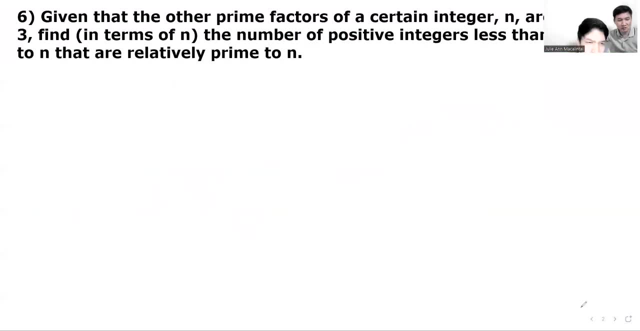 are relatively prime to the denominator 24.. okay, let's go to the next number, son here. okay, so six. can you put down this one? so i'll be the problem when you solve it. given that the other prime factors of a certain integer n are two and three, find in terms of n the number. 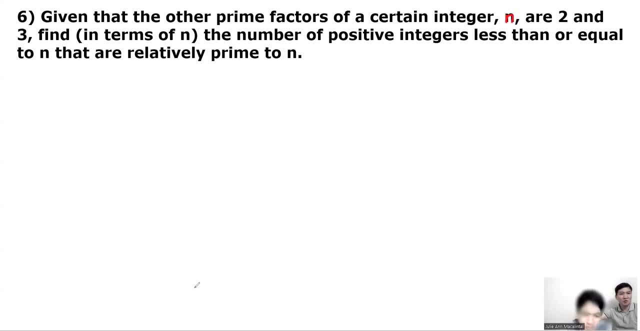 of positive integers less than or equal to n that are relatively prime to n in terms of n. no, this could. so this sounds intimidating, but Joshua showed you that this is uh quite, it's not very hard. yes, it actually is a simple problem to solve. so here, uh, it explains that there's. there's this integer n and r, uh, two and three. so it means 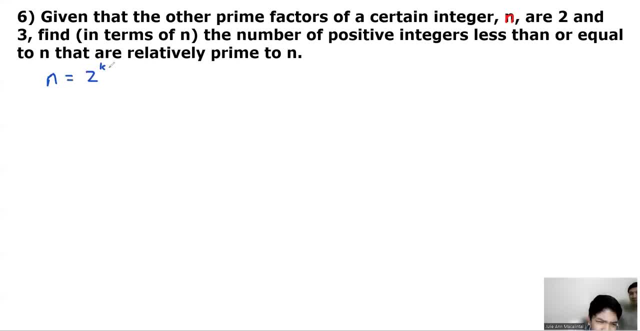 so the prime factorization of n is two to some some exponent. i'm not going to specify anymore because we don't know yet. yes, and then three. okay, so the number of positive integers less than or equal to n that are relative to prime to n, that's essentially the totient function of n. yes, so we just need to. 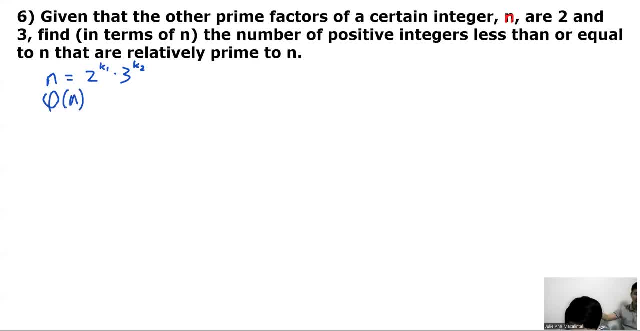 find the totient function. can you show us the formula that you will use so in the previous page? i'll just copy from this previous page. yeah, so you can use red. can you use red? okay, equals n times 1 minus 1 over p1, one minus one over p2, so on, so forth. 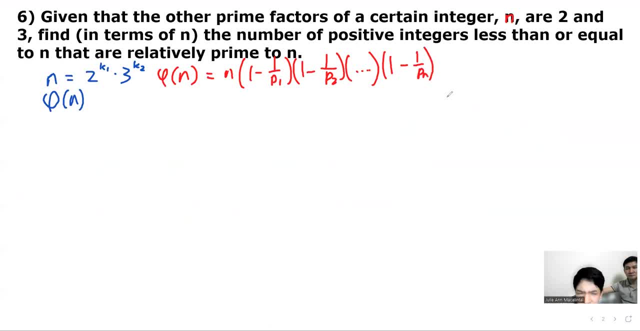 and then one minus one over p and, of course, the final prime- it has to end someday. the p: what are the yes p where all filter, all p, be all such bi, okay, right, well, the factors of n. you just remove that one, of course, or you invert this one, so it doesn't give me that problem anymore. 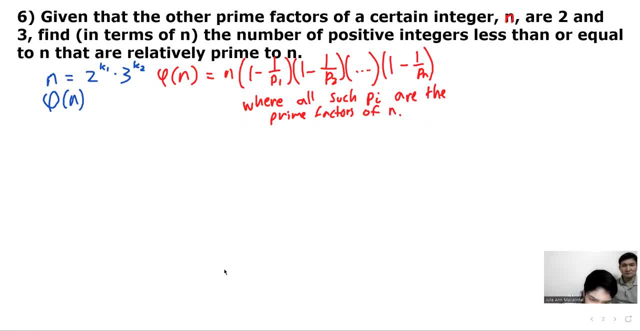 okay, so of course, we know that, uh, we know the prime factors of n, so that. so in this case there's two, three and then there are no other primes. there are no other prime factors. so we don't need to use this, this, this part. so essentially we just need to write down and write it here. 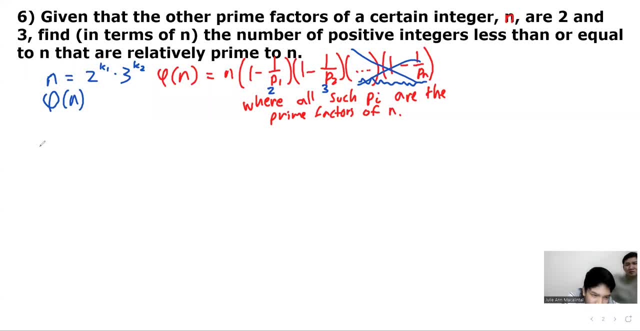 here. don't use that all that's the space to yes to utilize and then one minus one over like write everything. they're just the equal sign, the letter. you can think of our viewers as they're trying to learn. don't assume that they know already. yes, okay, so and of course, 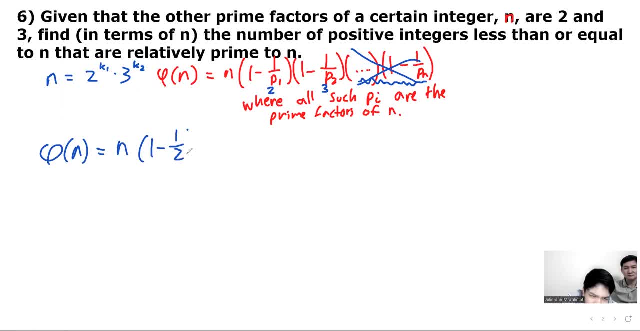 times one minus one over the first prime, two times one over one over one minus one over the second prime three, the second prime factor, yes, the second prime factor, three, and then simplify, cancel, cancel and over three, so such, uh, it has many words, but then it's not really, there's not really much to the problem. 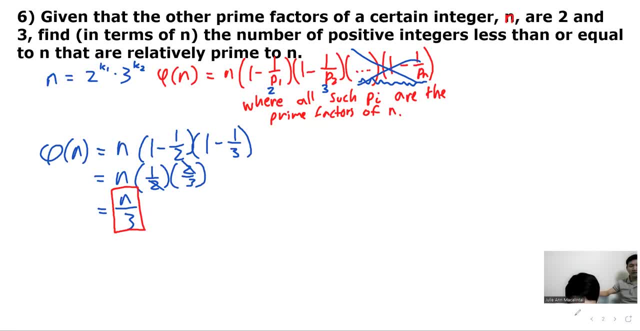 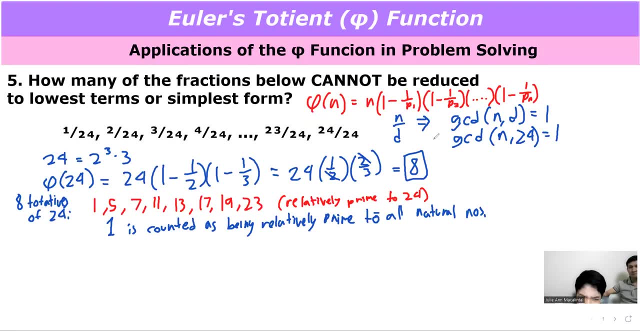 if you analyze it, the final answer is n over three. that's correct. so actually we can have. we have an example already of that. the 24 itself is uh has only two and three. and then guess what the, the quotient function of 24 is, that's uh, 24 over three or eight. yes, so we have. that's your, with your quotient function of 24. 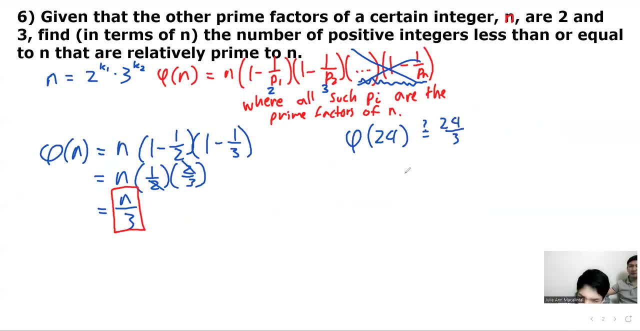 is, to this end, 24 over three actually is eight. yes, it seems they're the same. you're connected number six to number five. yes, so now we are moving on to the next problem. so now this problem is, uh, much more direct than six. but then this is: 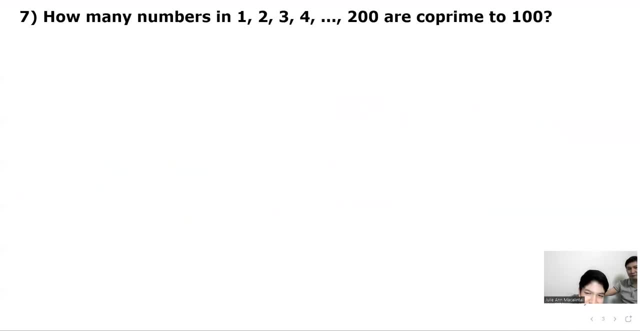 the most complicated of them. no, you just want to explain better. yes, this is simple, but the solution to get to the final answer is easy, but we just want to explain to our viewers what the everything means. okay, so. how many numbers in one to 100 are co-prime to 100? yes, okay so. 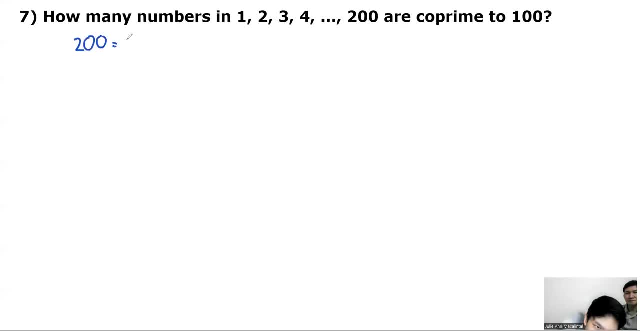 200. 200 is equal to 2 times 100. so therefore, obviously, because 100 is literally in the a factor- is a possible factorization of 200.. 100 and 200 cannot possibly be co-prime. okay, let's write down everything. so those: 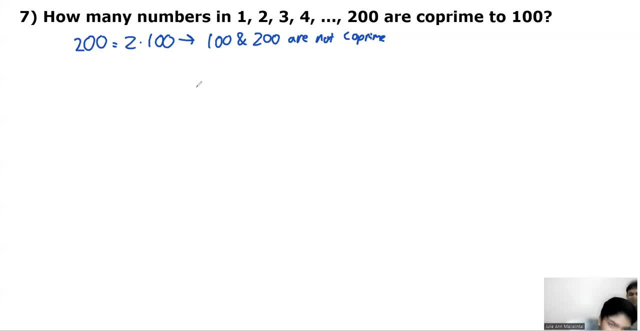 uh, viewers who want to bring. so, since one, 100 and and 200 are not co-prime, meaning yes, so 100 is not co-prime to 200. meaning they share, yes, they don't share it. yes, they share, they share, they share common factors. so, because of this, because of because 100 and 200 are not co-prime, it means all numbers. 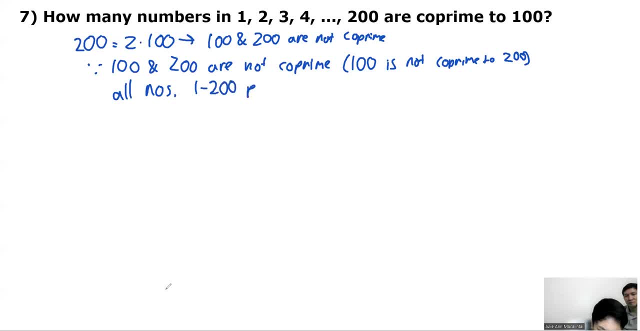 1 to 200. actually, this, this, this, not this, not this, this. that doesn't actually, doesn't actually prove that all numbers, all numbers- 1 to 200, co-prime to 200, are also co-prime to 100. yes, yeah, it doesn't. actually, you need to use the prime factorization: 100 is equal to. 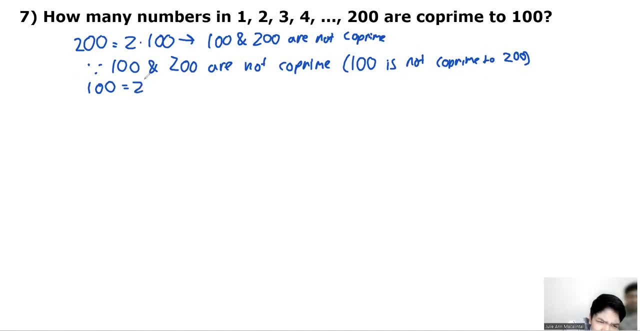 200 squared times 5 squared. 200 is also equal to 2 cubes times 5 squared. that they have the same, they have the same primes, they have the same prime factors. so then we can see that all numbers, 1 to 200 to 200, a co-prime, co-prime to 200. 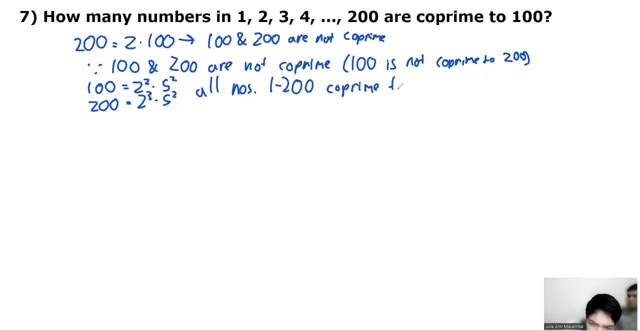 已經 200입니다- are also co-prime, are also. hey look at this thing: all co-prime, all numbers, co-prime, all numbers, co-prime. three spots to 100, that was 4 prime to 100? What do you mean? 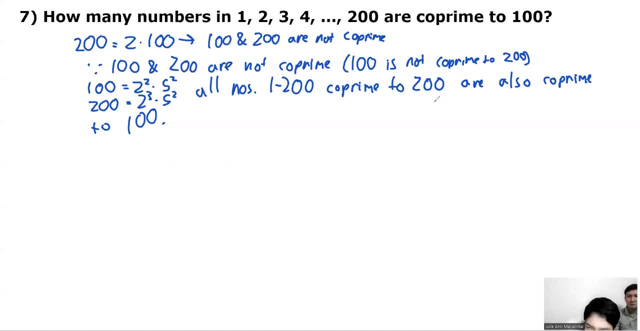 Ah, Typo 200.. Yes, Okay, So all numbers 100 to 200.. 4 prime to 200.. I did not notice. 4 prime to 100 equals 4 prime to 100.. Of course I did not notice. 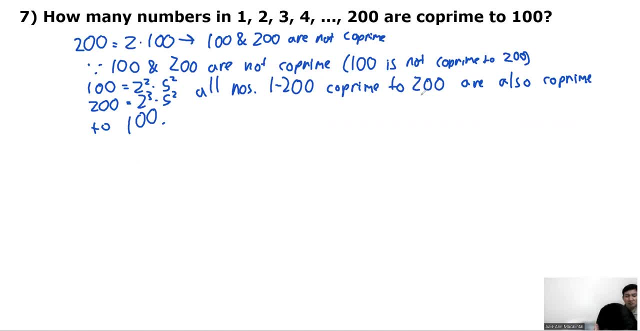 So be careful, Be very conscious. So 3 of 200.. Don't crowd all the numbers and the words. You have space, so make them nice. 200.. You can even use other colors to make to explain everything in. 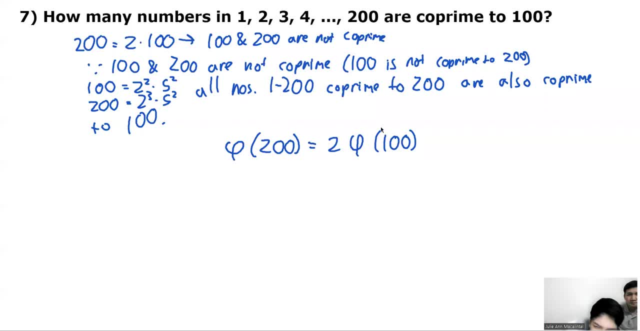 a well-fashioned manner. So on the right side and on the other side, you can, Yes, Okay. So we will just use again the same formula we used last time. We used it in 5 and 6. So I'll just put it here. 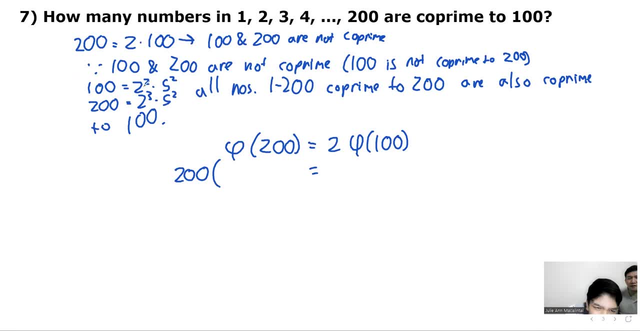 No worries, 200 times 2 directly. so we can explain this better: 1 minus 1 over 2.. 1 minus 1 over 5.. 2 to 100, 1 minus 1 half, 1 minus 1 5.. 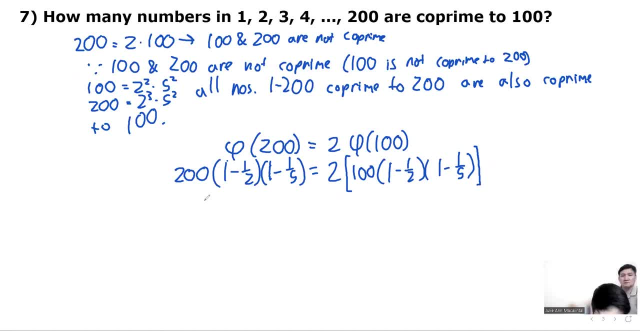 Yeah, So 200, simplify you. so you get 1 in half. So cancel by saying it twice 100, and then times one minus one-fifth of this equals two times one hundred times one half times four fifths. so we can cancel these two and then cancel that zero. 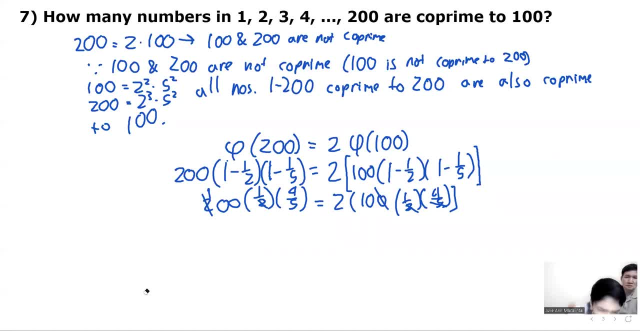 and use the bracket. okay, so eventually, one hundred over five times four. five is what twenty? so one hundred over five times four. twenty times four. twenty times four is equal to two times ten times four. so two times ten times four. that's basically the same. so it's the same: 80 so 80.. yes, of course, so there. 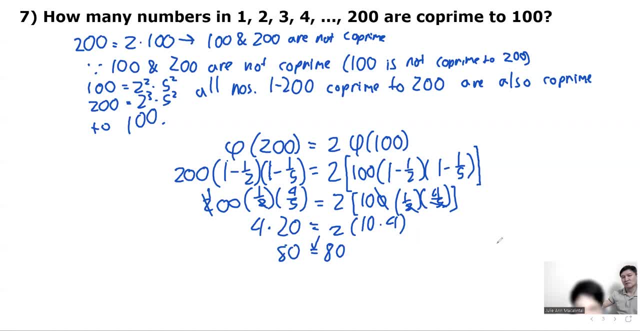 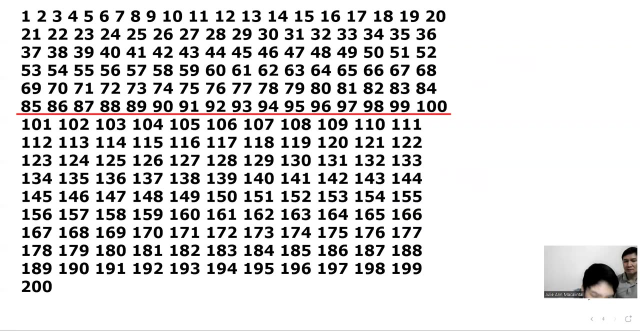 are 80 total things. there are 80 totals to 100, yes, from one to 200: yes. so what does this mean? so what? so i will just explain to them. explain it in words first: yes, so that we can, before we go to the next, to the flash page. 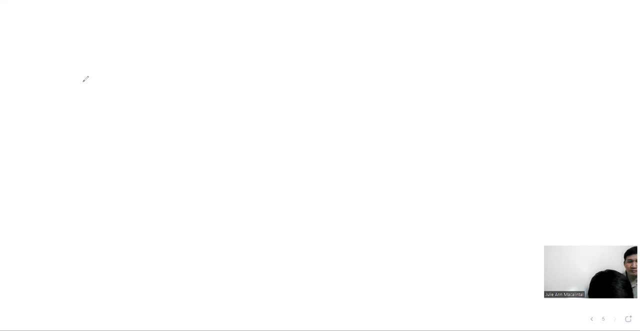 100 and 200 are not relatively prime. so yes, wait, let me explain this one. so the meaning is: uh, we have uh 80 totals. oops, meaning 100 and 200 are are not not. sorry, are not. can you give me some excuse me, can you? 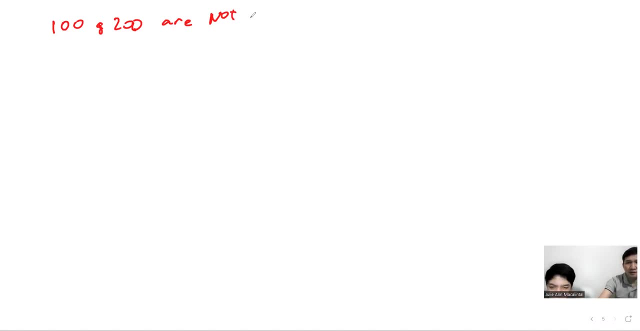 it's not relatively prime, meaning they have common factors or divisors. you know, since the prime factors of both 100 and 200 are exactly the same, which are the prime factors two and five, when looking for the totatives without change the power- sorry, let me just say we're looking for the 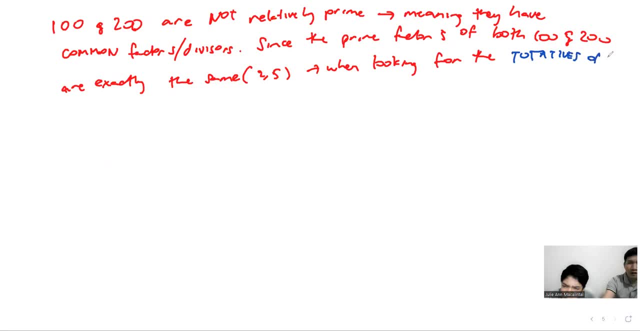 totatives of 200 with a total function of 200, meaning that we're not widening the value of 100. we'll just say 2 over 0 is negative because we know that the positivelines arearning the positive integers less than or equal to 200. 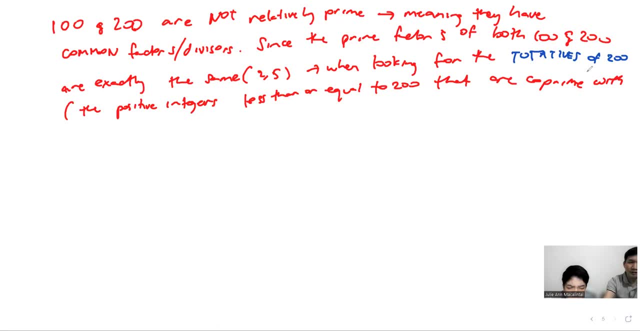 that are conscience and the transferable 2 primes written. You simply have to do exactly the same as how you found the totatives Of 100.. How? By? By crossing out 1. By crossing out the 2s and 5s. I will just demonstrate that a little bit later. 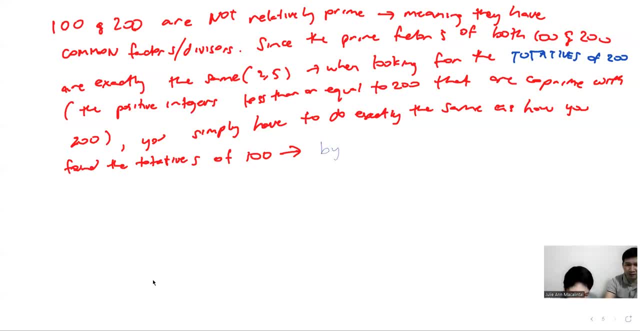 By- I'm sorry- The 9 sides, By crossing out all the multiples of 2 and 5.. We just need to need to extend beyond 100.. Up to 200. So essentially all of the multiples of both 2 and 5, they just all share the same totative table sort of. 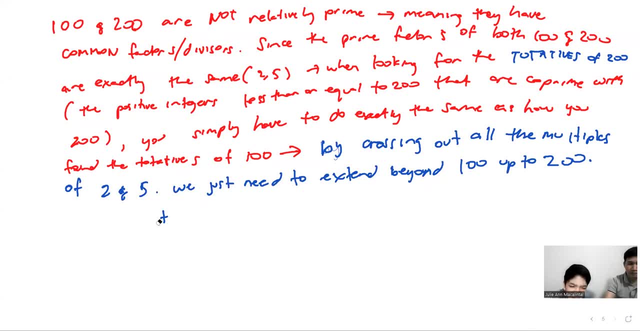 Yes, They're just at different lengths. So here, as Joshua pointed out, we're going to demonstrate such a Oh, yeah, Okay, Yeah, I will just. Oh, can I write here Thus, when we cross it out like that: 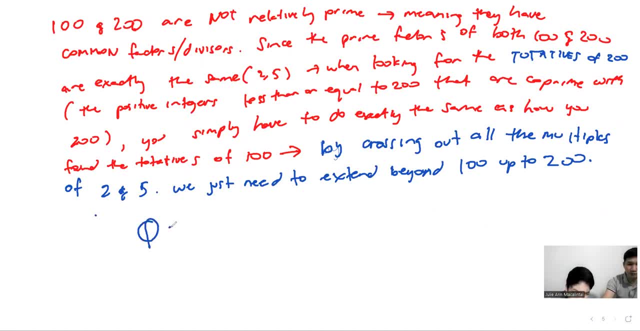 the totatives of 100 is 40. Then the totient function of 200 is 2 times 100.. Correct, Yes, So this will be 2 times 40, which will be 80.. So, Joshua, can you demonstrate to us here? 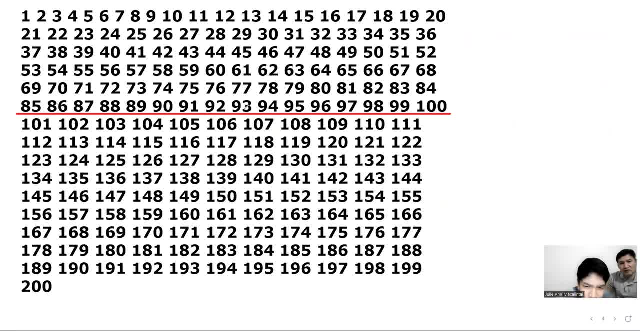 We will really get 40 for the first 100 and another 40 from 101 to 200.. Okay, So let's cross out all the multiples of 2.. Is this your single length? It would be very visible from the. We'll try all the multiples of 2 that Joshua is crossing out. 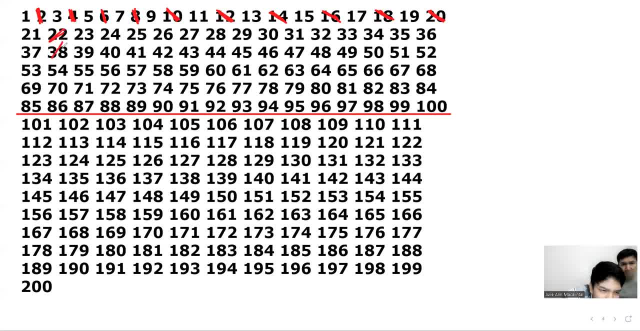 I'll just make a Yes. Yes, I will use that pattern. Okay, So I'm just crossing out the multiples of 2. Then we will count if there are really 40 left after crossing out all the multiples of the prime factors or divisors of 100. 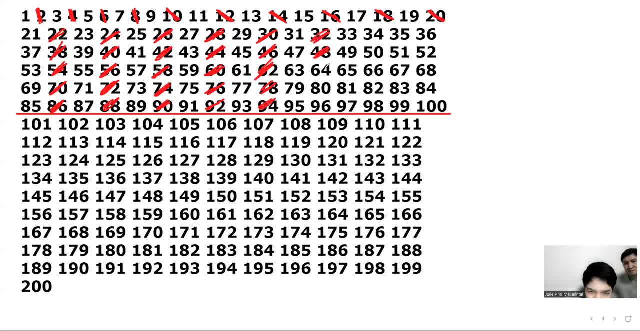 Let's see, buddy. Okay, Let's see if there's a 50. Yes, So how about the Multiples of 5.? Multiples of 5?? Use the blue, Just like the Like blue. Yes, 5,, 10,, 15.. 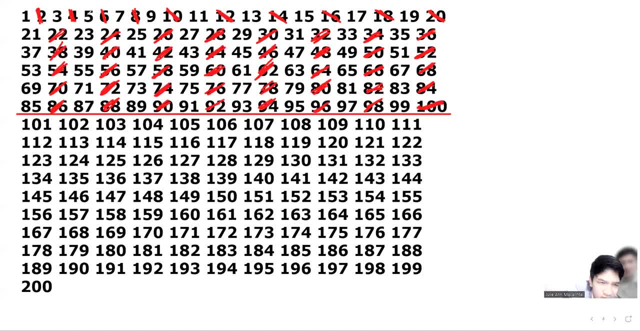 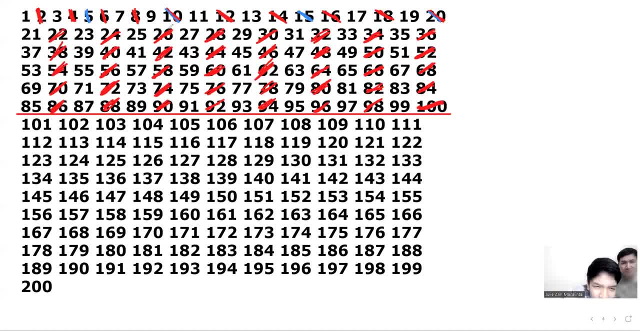 10. 10. 10. 10.. So they repeat when Just cross them outside. They don't repeat regularly, They repeat regularly. but then how it's written here on this table? Sorry for the Ah. yes, they form a pattern too. 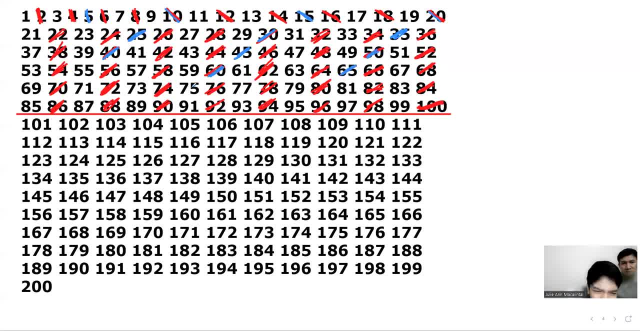 They go like this, They go diagonally. Aha, Okay, Okay, Okay, so One hundred, Ah, yes, one hundred. I almost forgot one hundred itself. They cross out anyway, so let's count. They are, You say, yellow. 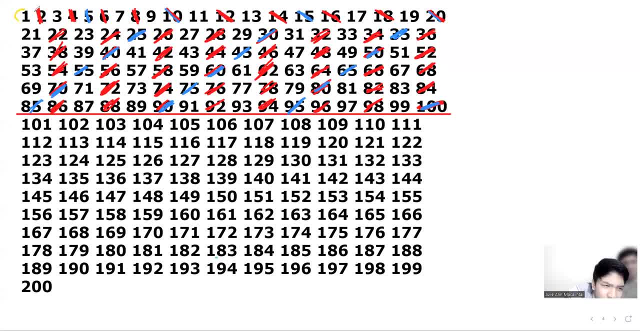 I say yellow: One, two, three, four, five, six, seven, eight, nine, Ten, Eleven, Twelve, Thirteen, Fourteen, Fifteen- I'll just go down some more- Sixteen, Seventeen. 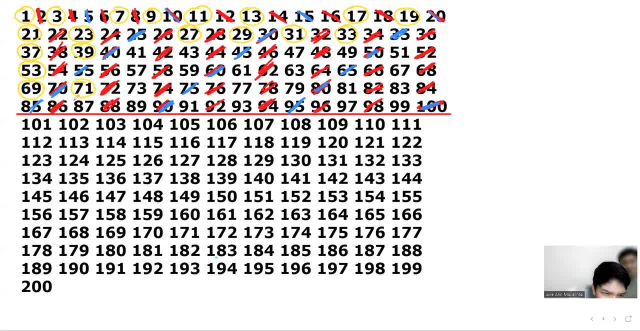 Eighteen, Nineteen, Twenty, Twenty-one, Twenty-two, Twenty-three, Twenty-four, Twenty-five, Twenty-six, Twenty-seven, Twenty-eight, Twenty-nine, Thirty, Thirty, Twenty-one, Twenty-two, Twenty-three, Twenty-three. 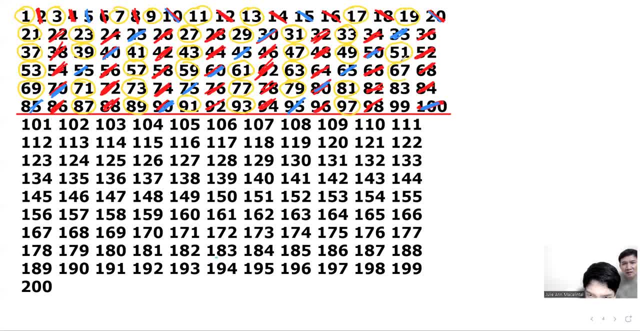 Twenty-four, Twenty-five, Twenty-six, Twenty-seven, Twenty-eight, Twenty-nine, Forty, Forty, exactly Forty, indeed Totatives, Okay. so now the Those forty are, Yes, Relatively prime to one hundred. So now let's. 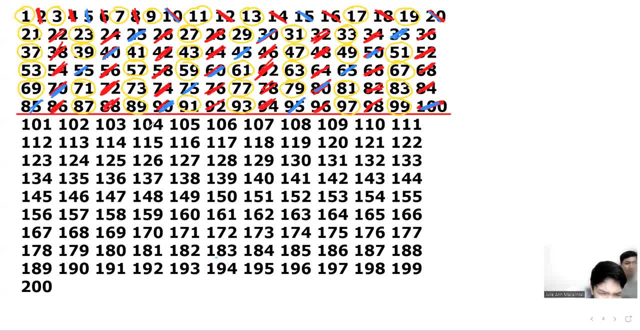 So now the Let's do from one hundred to One hundred and one to two hundred. Yes. So now the twos. now go directly, diagonally. Yes, Yes, Yes, Along the way, Yes, And then also do the fives. 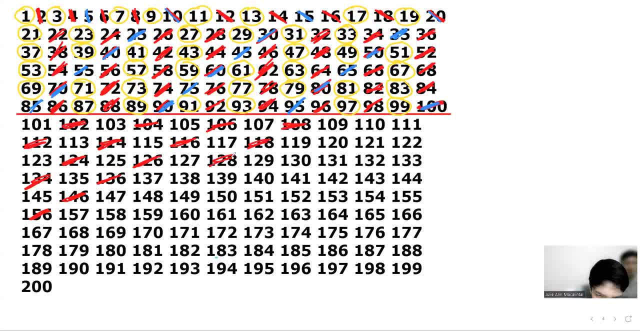 And then just spot them. Yeah, Let's do the twos first, And then multiples of two, From one hundred and one to two hundred, And then here we are trying to demonstrate to our viewers the meaning of the solutions for the Euler's Toshin or phi function. 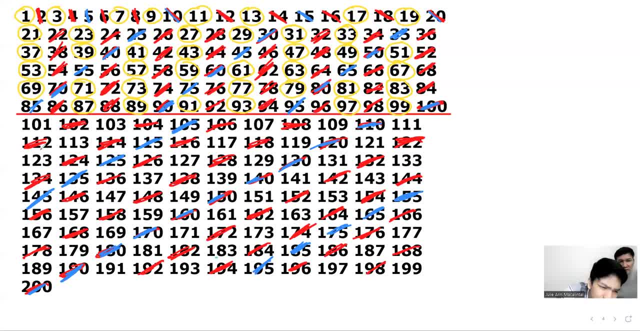 okay, so let's count again. how many are co-primed to 100? yes, which are also co-primed to 200, the outside the 100 boundary now. okay, so one, two, three, four, five, six, seven, eight. let's go down there, because this one was left out. 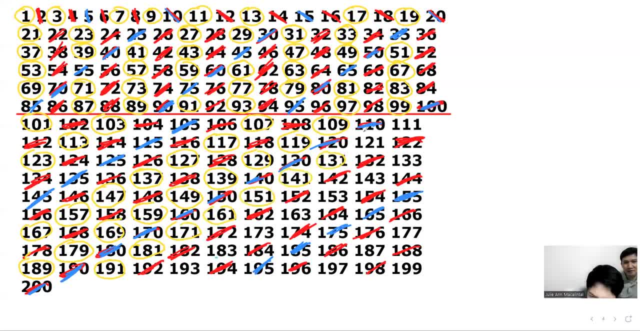 five and six and seven, three: 30, 31, 32, 33, 34, 35, 36, 37, 38, 39 and 14. indeed there are 40 coprime numbers to 100, which are also co-primed to 200. 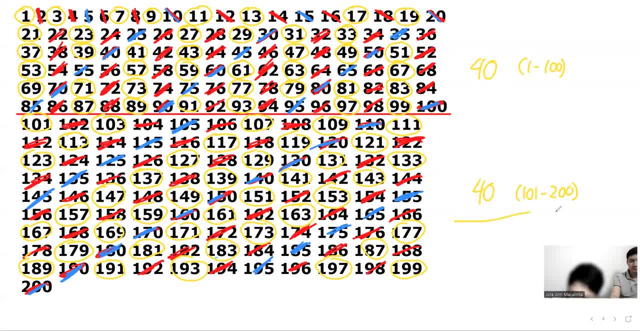 100. this one is 101 to 200.. so now we're going to find out how many are co-primed to 200,. okay, So now, in total, that's it 80.. 1 to 200 in total. 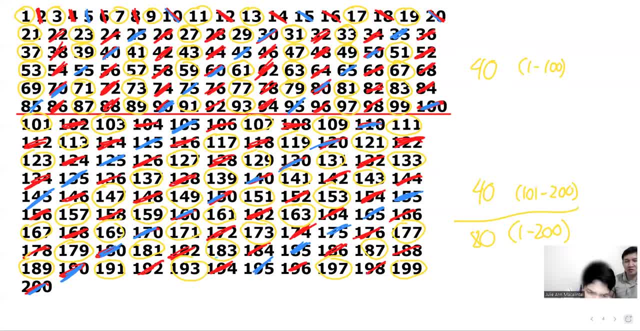 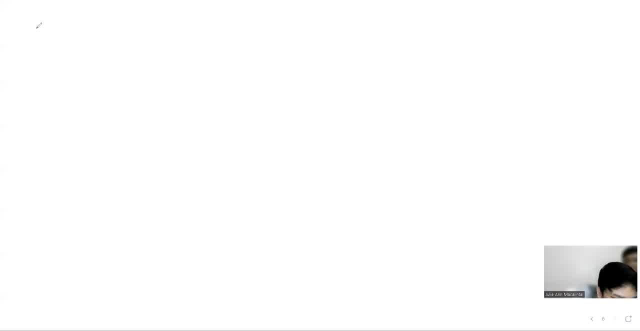 That's really true. So can you show us alternative solutions to this problem? Yes, So this alternative solution is again based on the dark blue, again It's based around the prime factorization. So 100 is 2 squared times 5 squared. 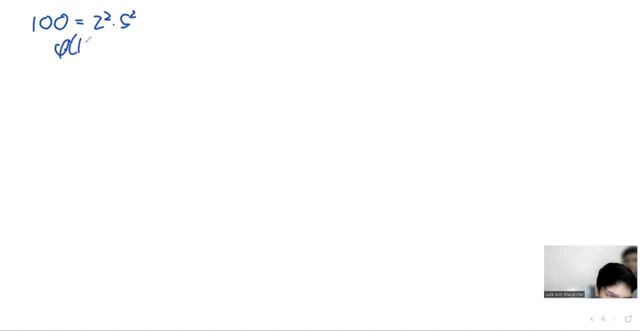 So the phi of 100, we can manually calculate, That is, since it's only composed of powers of 2 and powers of a prime, another power of a prime, and they're both multiplicative. Actually, there's a hidden step here. It's not readily shown. 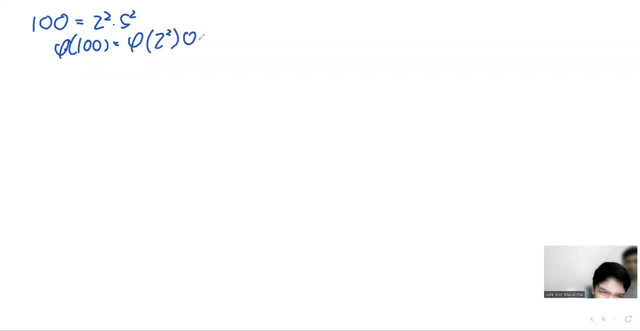 It's actually phi 2 squared. It's phi 2 squared times phi 5 squared. So then that is equal to our special formula for perfect powers of primes. So 2 squared minus 2 to the first, 5 squared minus 5 to the first. 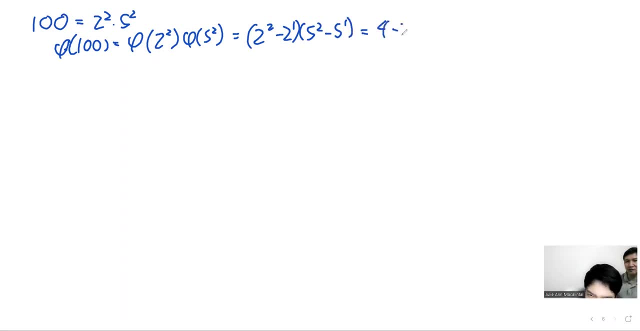 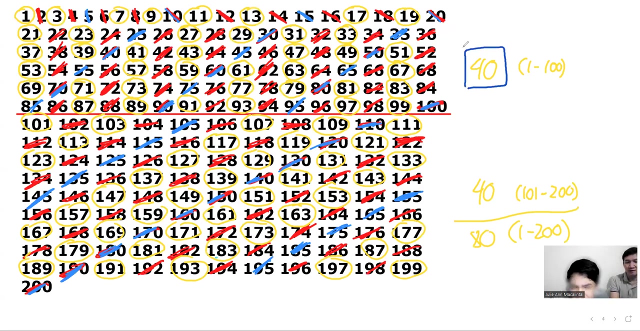 Yes, So then that is equal to 4 minus 2.. 25 minus 5.. Equals 2 times 25.. So that's equal to 40.. Yes, There are 40.. We saw in the previous page- can you turn the page, Josh? that there are 40 co-prime numbers to 100, from 1 to 100. 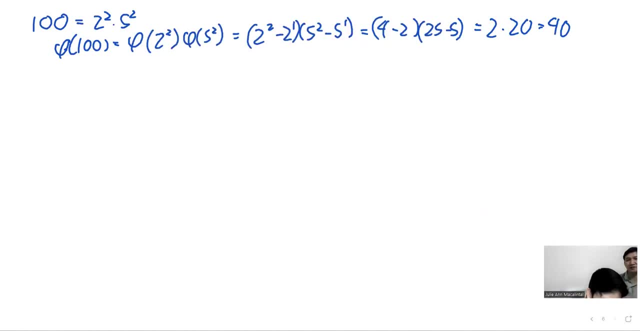 Ah, okay, So 40 totatives of 100, meaning there are 40 co-prime numbers, Or those numbers which you can share any common factors with 100, from 1 to 100.. Correct San Yes. So now there's a special: there are 40. 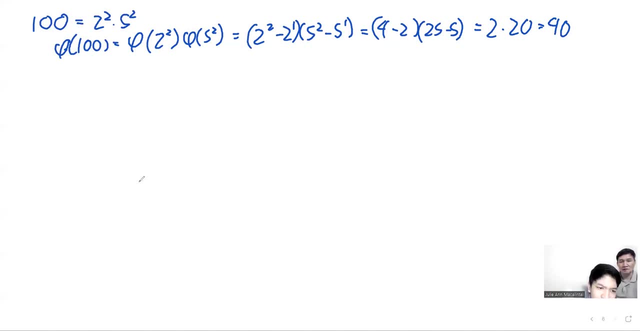 So there's a special property involving GCDs, So that such property is: Can you show me the color, Sure GCD AB. Can you give us an example? There's this property? Yes, I will give an example. 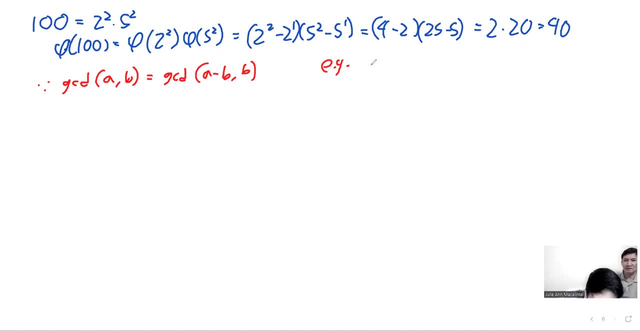 So it's the same. Exempli gratia means literally, for example in Latin, 32 times 4.. A- B, Okay, So then GCD: A minus B, So that is 32 minus 24 B. 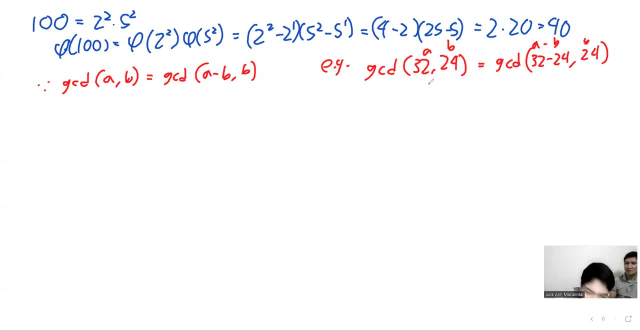 So that's just 24.. So let's see. So 32 and 24, the greatest, No GCD. I'll just put it again. I don't want to simplify GCD of 8 and 24.. 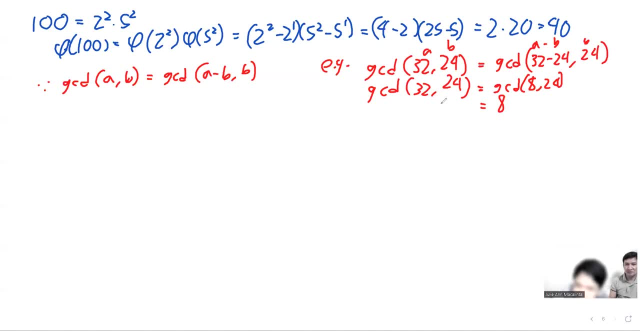 This right side is easy, That's just 8.. And then the left side, that's also 8.. Yes, It's happened. So, yes, So this formula is true. We will use this. Joshua will use this formula for solving for this and proving this one. 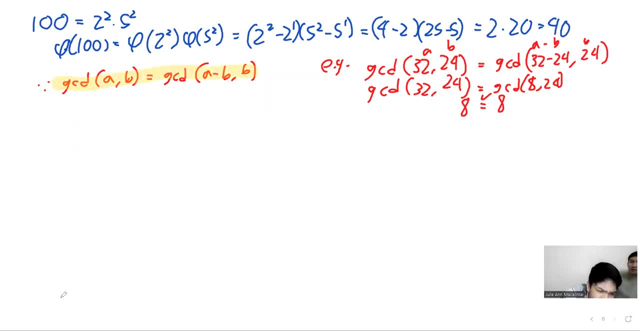 So we were saying all numbers which are co-prime. This proves the fact that This will prove the fact that the numbers co-prime to 100 are also co-prime to 200.. Yes, This will explicitly show that not all such cases. 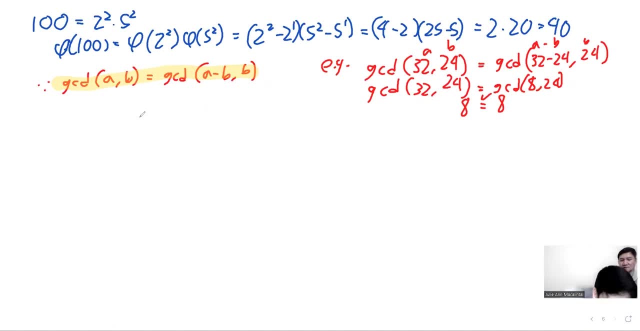 Yes, So the GCD of cosine is. So this is like dark green. Okay, Dark green GCD of 101 and 100 itself is equal to GCD 101 minus 100.. So GCD is just 1.. 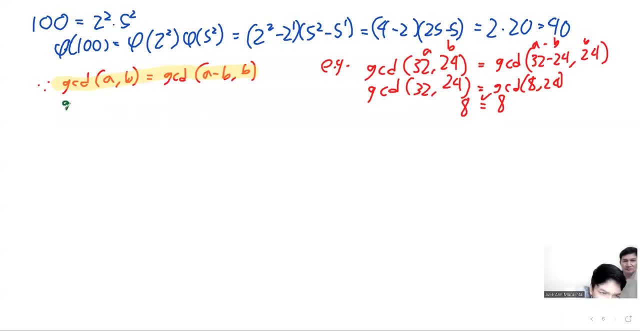 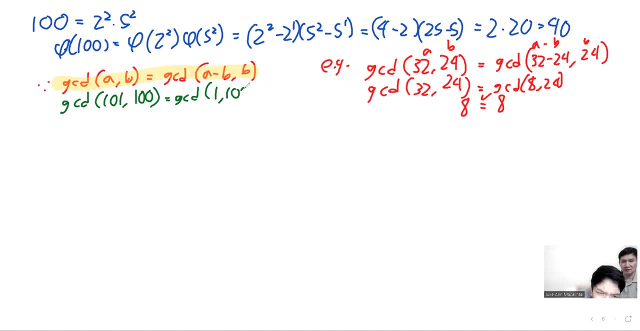 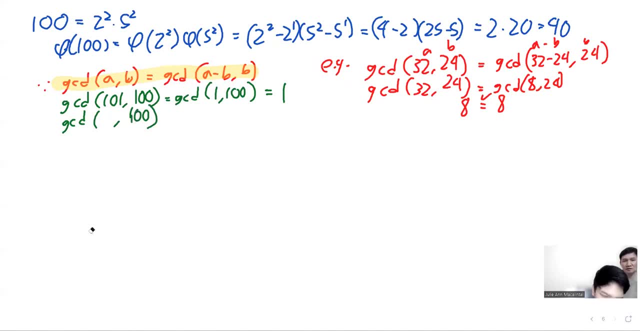 Yes, So. And JCD2, 100.. Oh 102.. Oh 102.. Oh sorry, Oh sorry, 102, 100 is equal to GCD2.. So that is equal to 2.. 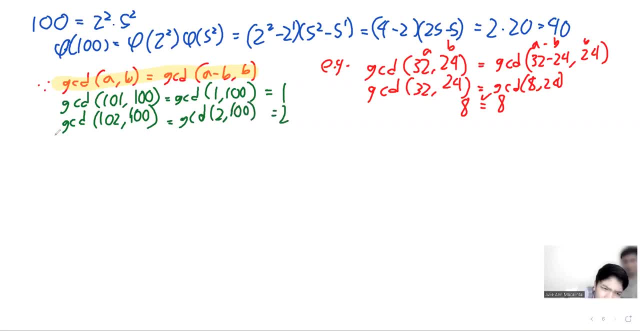 And then GCD103,. 100 is equal to GCD4.. So 102.. Oh no, Oh sorry, My name is Connor, So let me open the box first. Shannon, Yeah, Okay. Okay, to gcd 3: 100. so that's just equal to 1. 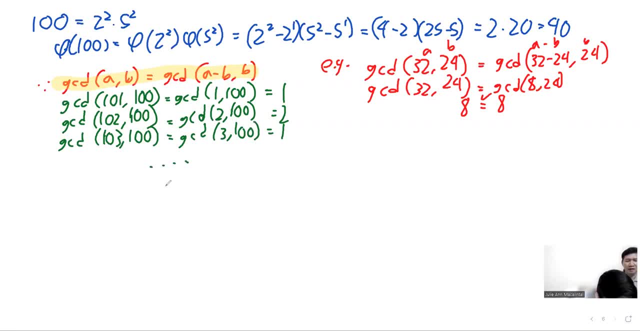 can i do it up to no, up to 106, just to prove that this really, this formula really works. so see: gcd of 104: okay, 104, 100 is equal to okay. gcd for 100, which is, which is equal to two. oh wait, is it four? four, yes. 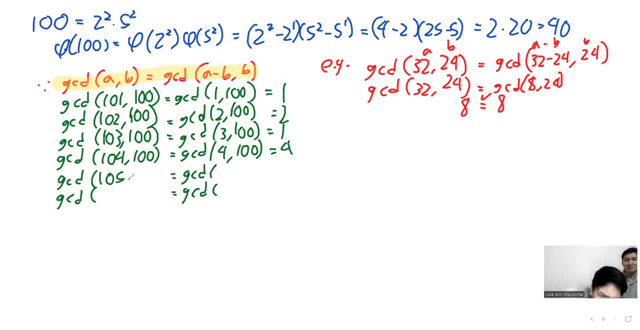 okay, yes, okay, okay, yes, okay, yes. so 105, so 105, so 105, 100, 100, 100, five, five, five, one hundred five, better, one hundred five, better, one hundred five, better five, five, five. go to five, yes, and then one oh six. go to five, yes, and then one oh six. 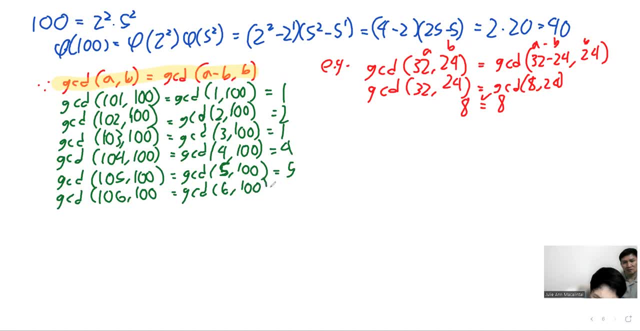 go to five, yes, and then one, oh, six, one hundred, six, one hundred. that is one hundred, six, one hundred. that is one hundred, six, one hundred. that is, this, is, this is, this is yes, all the way, go down. what if you? yes, all the way go down. what if you? 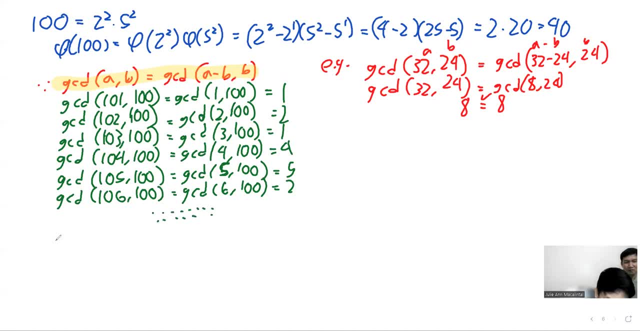 yes, all the way go down. what if you just proving this one? it will go up to just proving this one, it will go up to gcd of 200 and 100. applying this formula has the same gcds: 100 and 100. ah, so this, this, literally. 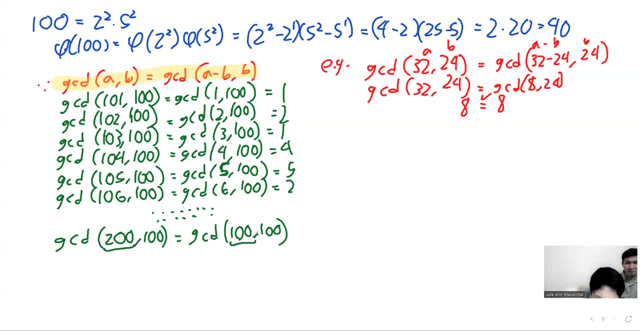 shows the proof that we were claiming earlier: 100, the the ones that are pro prime to 100. they are in fact co-prime to the one, the other extent, the extended family, sort of so meaning the numbers co-prime to 100 are also co-prime to 200. yes, not from 200, they're also. 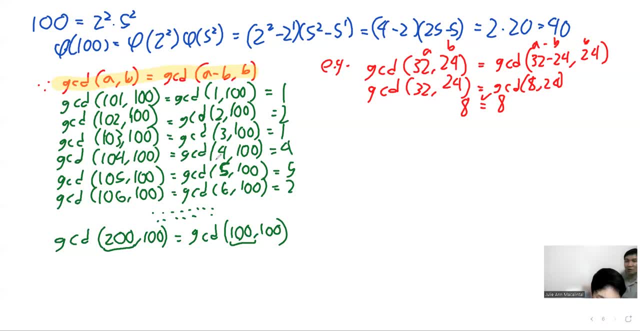 co-prime to 100. yes, all the numbers, 200 are co-prime to 100. yes, so this is 100. yes, so they have exactly the same prime factors. and then 100 happens to be inside the prime factors of 200, so 100. 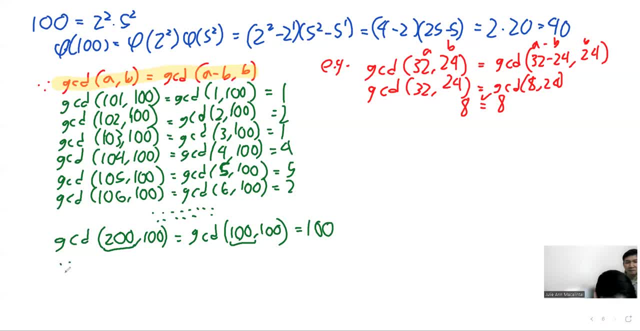 so there are, since there are, there are, there are 100 fee. i said that, uh, fee 100 is equal to 40, 40, as we've seen above, 40 co-prime is equal to 40, co-prime members numbers to to one hundred. 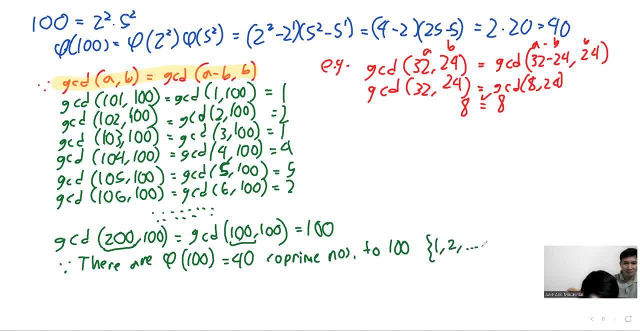 one hundred one hundred. this is the set from one. this is the set from one. this is the set from one to to to vital, vital, vital, 100, 100, 100. so these are, so, these are, so these are. can you transfer that? can you transfer that? 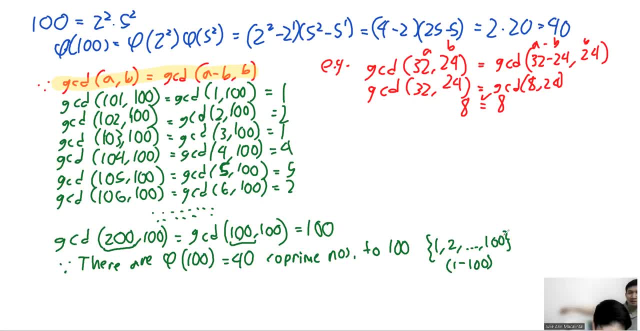 can you transfer that? does, does, does that? So there are also 42 co-prime numbers. We can see that they are exactly the same numbers because they correspond to 100 in the set from 101 until 200.. This is 101 to 200.. 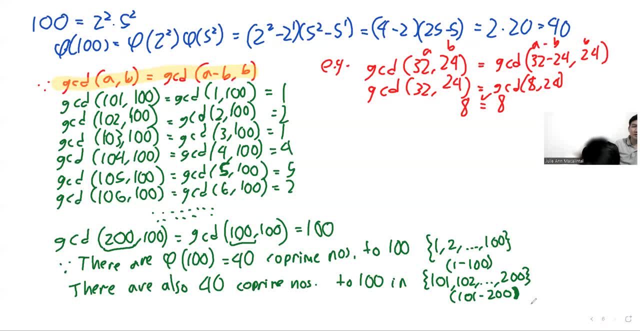 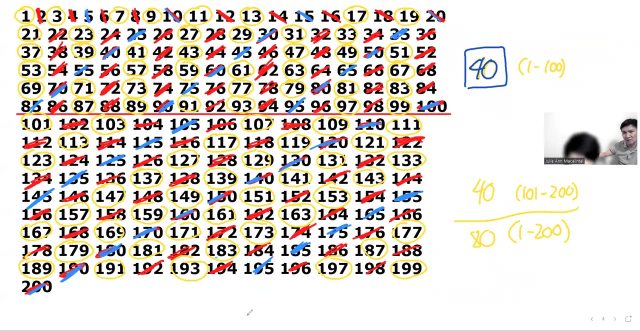 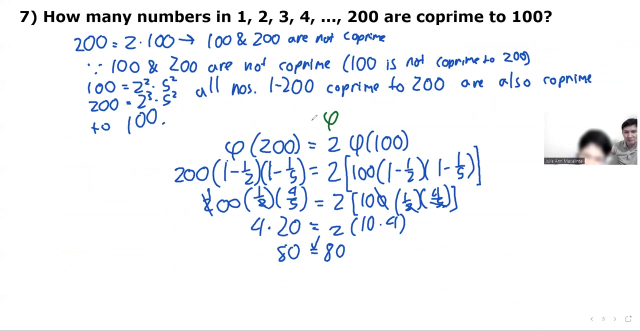 So, in short, how many in all? in all, in total, Of course, 40 plus 40 equals 80.. Once again- this is the side note here- The phi is multiplicative, so eventually, phi of 200 will just be phi of 2 times. let's. 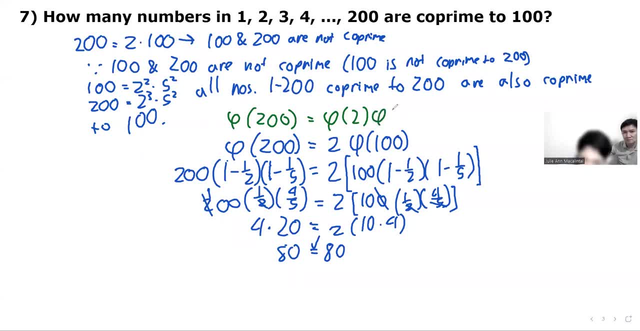 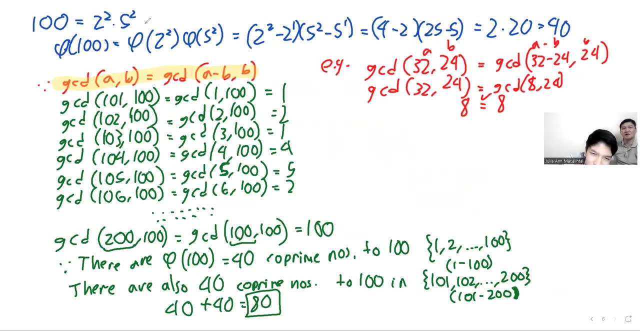 just move this Phi of 100, so that's going to become 2 times phi of 100. Right? Yes, So this has 2 times 40.. Yes, So it will be 80.. Yes, And another. last but not least, can you turn to the next page?